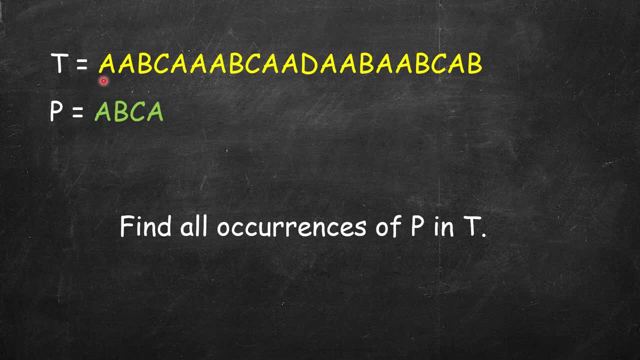 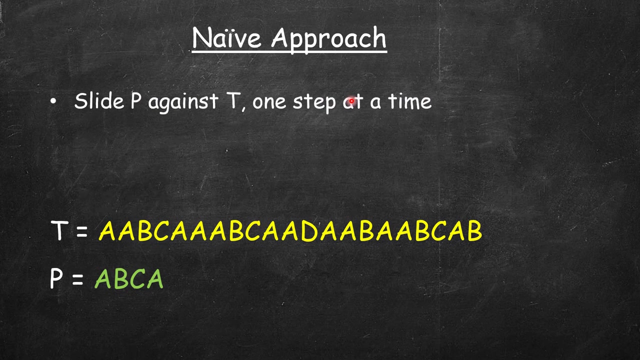 So if you are asked to do this, that find ABCA in this, all the occurrences of pattern P in the given text T. So if you are asked to do this, that find ABCA in the given text T. So if you are asked to do this, that find ABCA in this, all the occurrences of pattern P in the given text T. So if you are asked to do this, that find ABCA in this, all the occurrences of pattern P in the given text T. 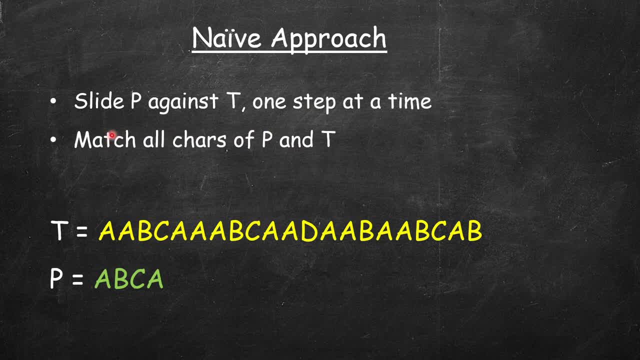 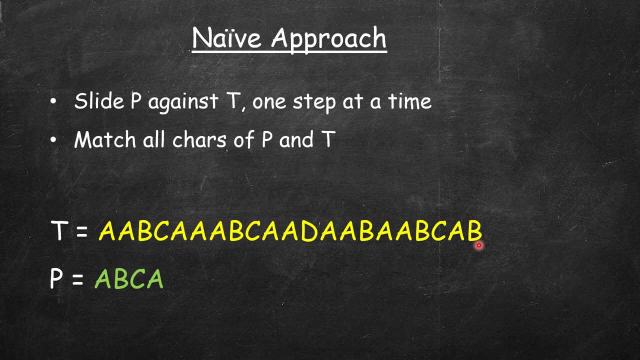 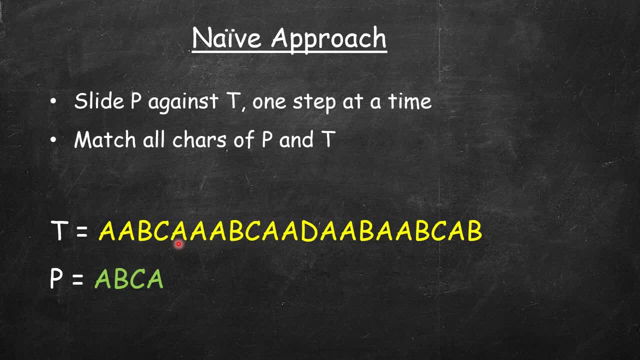 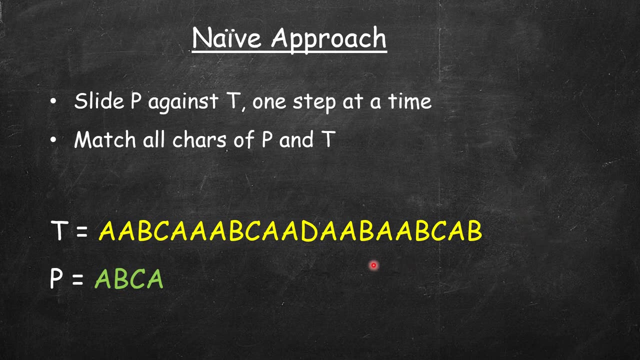 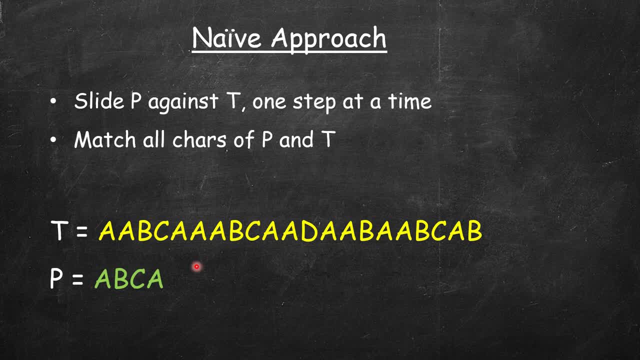 reduce this time complexity from o mn to o of m plus n on average case and in general cases. but there is still one worst case and we will see that later. but in most, the most of the practical cases, it will be o of m plus n, assuming we how we calculate hash. in this case we will use a. 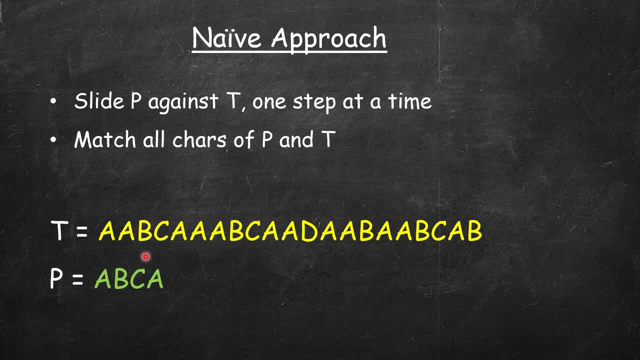 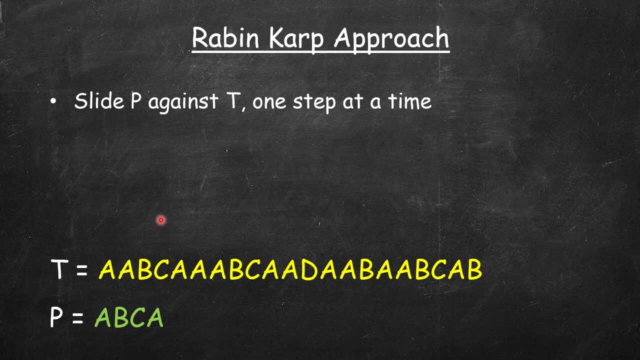 rolling hash. so we will see. we can calculate the hash of a window in constant time. so now let's see the Rabin-Karp approach. so we slide p against t one step at a time. same as the naive approach. but what differently we do instead of matching p against t. so matching p against t means comparing. 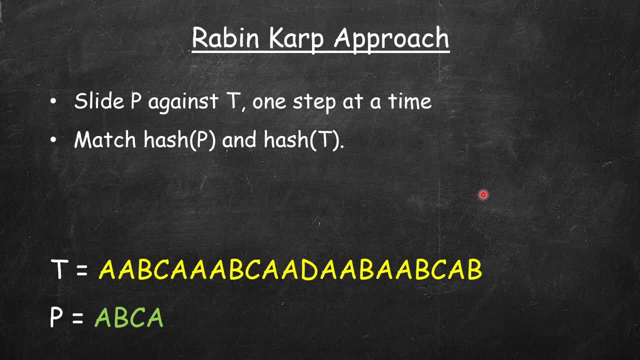 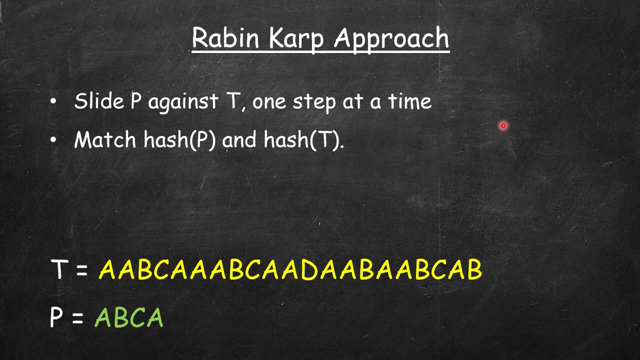 all the characters so it can be o of m time in naive way. but here we are comparing a value. hash of p is a value, integral value. hash of t is also a integral value. so here t does not mean hash of the component complete text, just the current window in the text comparing that is constant time. so provided if we 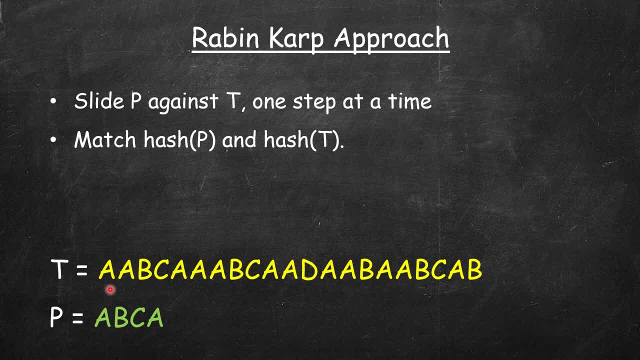 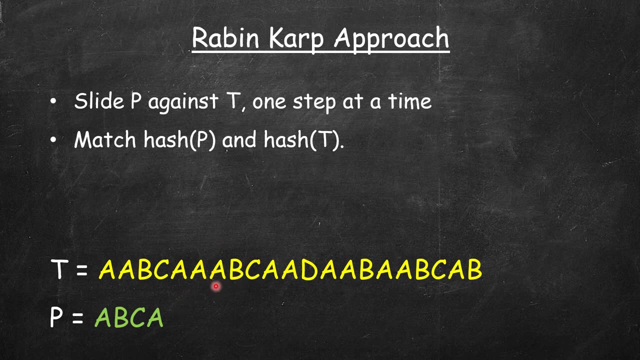 can update the hash of next window from from the previous hash. so if we have hash of four characters and then we have to move it by one step, you will notice that just one character has changed. so these three character will remain in the next window. also, first character will go away and one 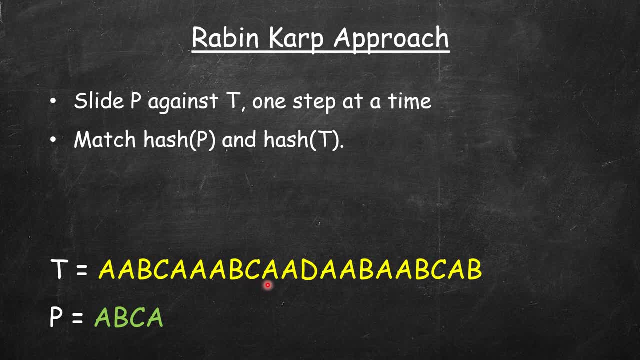 character will go away, and then we have to move it by one step. so we have to define our hash function in such a way that it is sum of character multiplied by some constant, plus next character multiplied by some constant, so that we have a value. in the next step we will subtract one value. 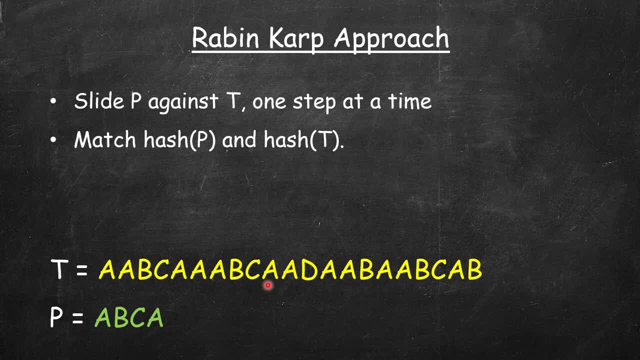 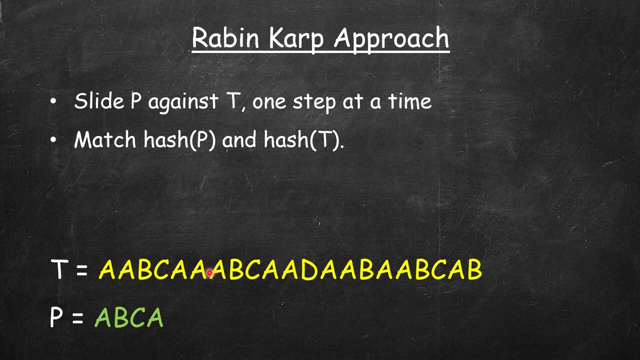 and we will add one value. so this we will call rolling hash and we will see how we will calculate that. so once we match, are we sure that if the hash matches, then, uh, the pattern and text is also same? no, it does not. if your hash function is very, very good, then the chances that two 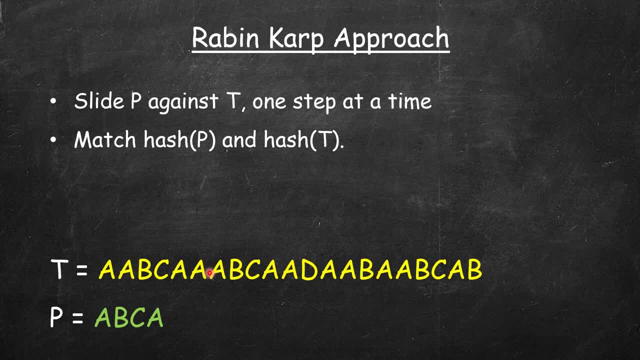 different strings will have a similar hash will be less but it will not be zero. if you have a really poor hash function, which we will see an example, then there will be many, many more collisions. so just matching of hash does not mean the pattern and text has matched. so once there is a match- if 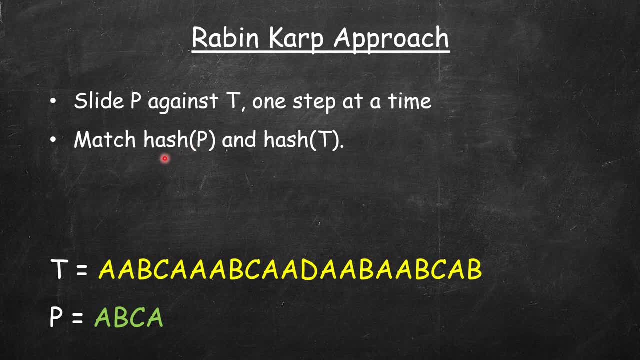 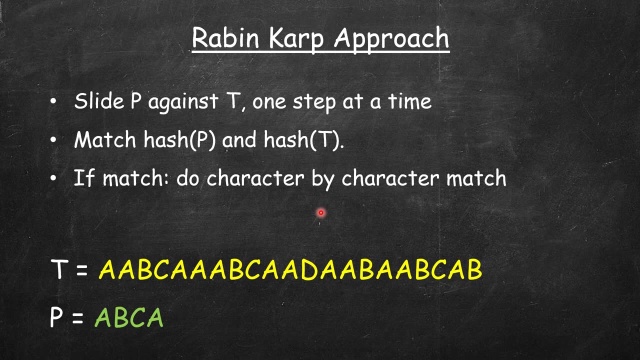 there is no match. there is no chance of strings matching. but if the hashes match, then there is a chance of match. so next will be: if there is a match, do character by character match. so on average case we will have to do it a few times. let's say there are five occurrences of this pattern in the 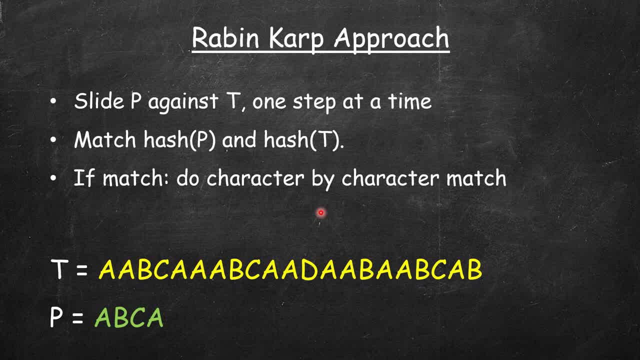 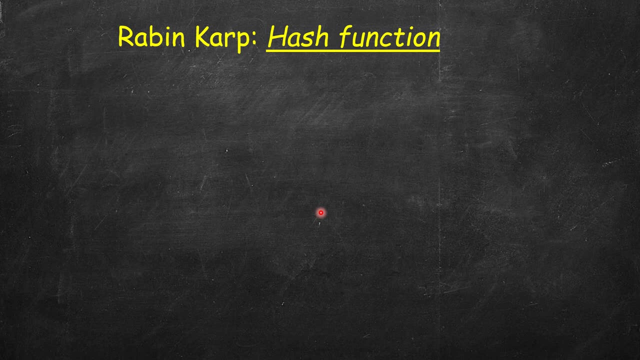 text. and let's say hash is matched six times. so one time it was a false positive. so on average it will be five times m plus n. now we have to talk about hash function. a lot, lot of it depends on hash function. main logic lies here. so let's say we have a text c1, c2, c3, all the way up to cm. so 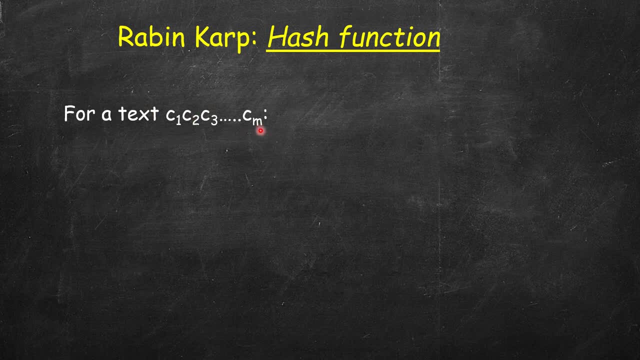 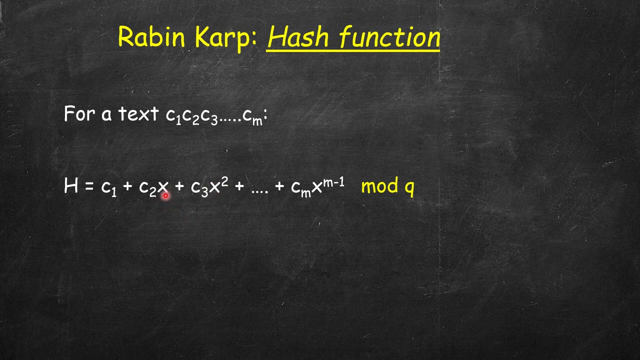 there are m characters in this text and c1, c2. these denotes the characters. so we will define hash function in this way. so c1 plus c2 times x. so x is some multiplier which we will see. generally we take some prime number. so c1 is the character. so by 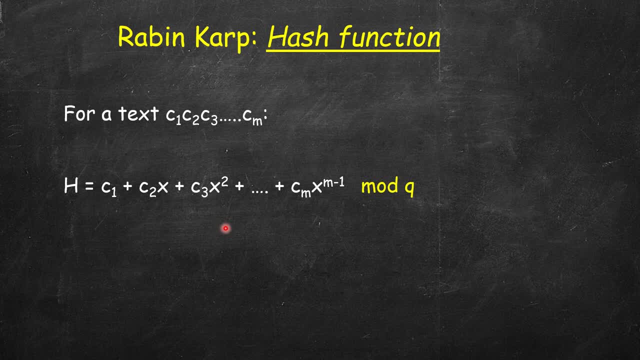 character we mean the sky value of this character. so for example, a sky value of capital: a, 65 small 8, 97 small beats 98 and so on. so first character, then second character, times c2 x plus c3 x, square, all the way up to cm x, m minus 1, and we will be taking modulo. 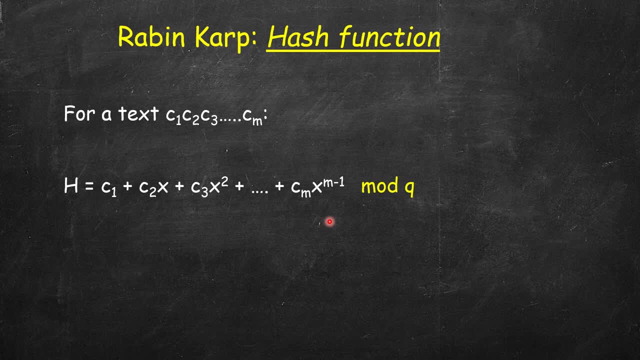 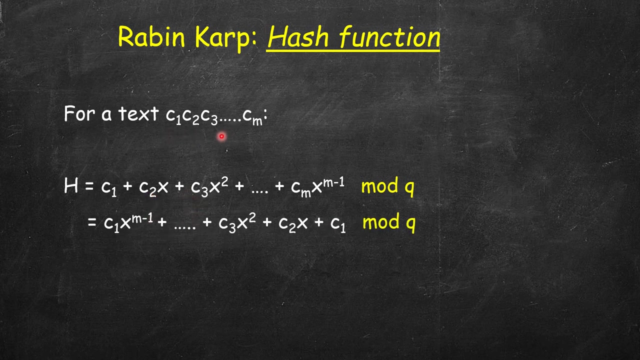 some number, because this can really become very big and it can overflow and you, after overflow, you may not get the desired result. so we keep taking modulo some quantity so that it's within some range. this is same as this, exactly. this is not same as this, but let's say we have 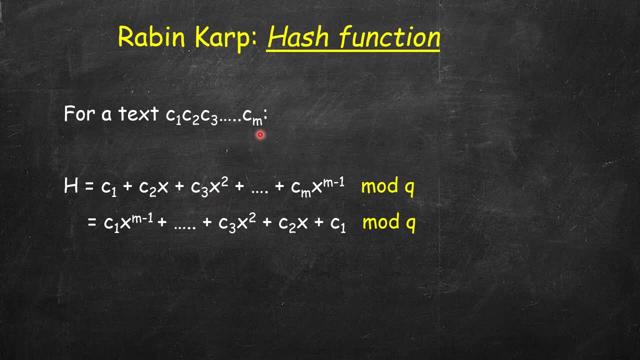 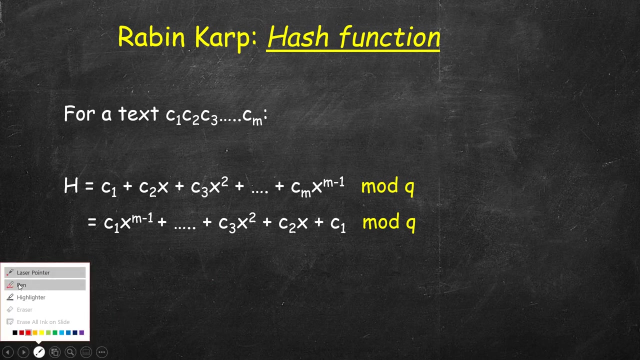 this text. nothing stops us from taking c1. actually there is a mistake here. uh, this should be uh c1 next to this is fine. then it should be uh cm. so let me correct it. so this is cm. the last one. this is c, m minus 1. 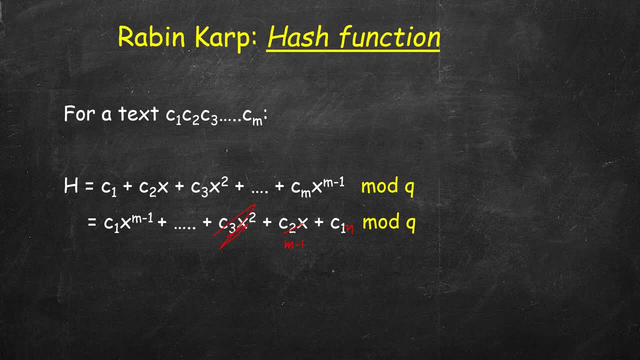 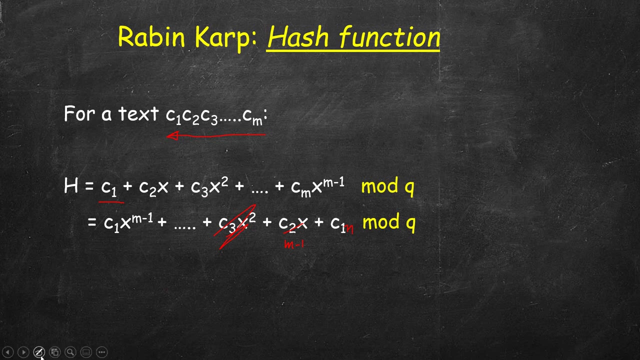 this is cm minus 2, so let's forget it. so instead of multiplying here x, 0, then x, we have done it in just reverse order. so nothing is so. this is as good hash function as this one, and we can use them in different scenarios. so let's say our window is, we are sliding window from left to right. 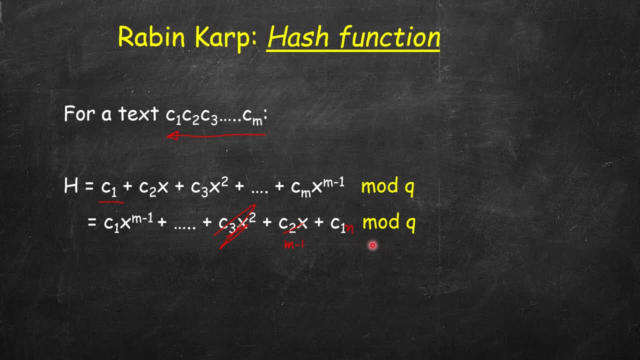 then the second one would be more efficient, calculating it in constant time from the previous hash, and if we are sliding the window from right to left, finding the pattern, nothing stops us from sliding the window from right to left. so in that case we will go with the first one. so we will see why it is easier to use the second version. 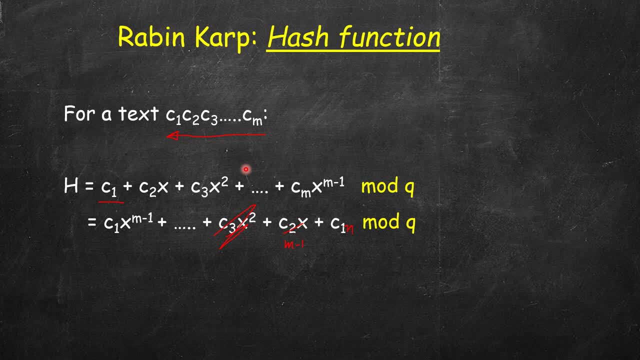 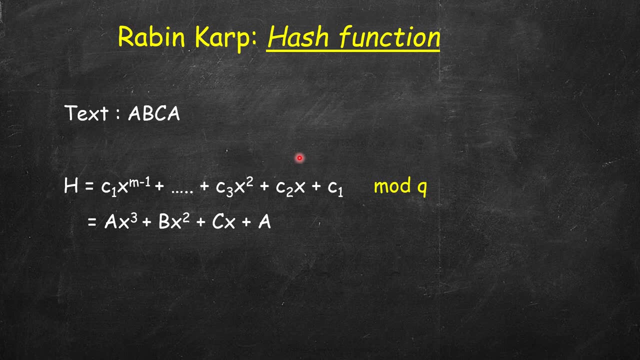 when we are sliding from left to right. left to right sliding window is quite natural and we will use that next. let's take an example. so we have a, b, c, a, a concrete example. this is the text for which we want to calculate the hash function. so, again, i had copied it. so again, this is a mistake. 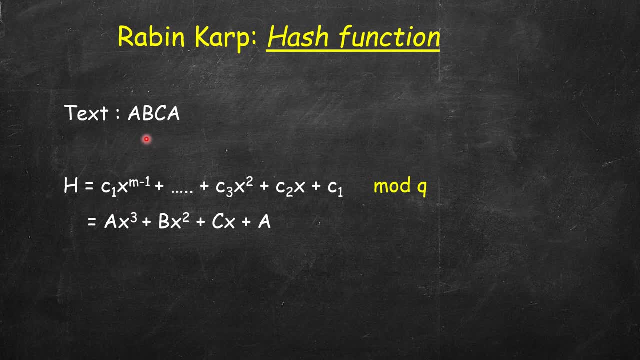 so, uh, first character, so m is here four. there are four characters in this text for which we are calculating the hash. so first character multiplied by one less than m. so you see x, m minus one, then b, x square, c, x plus a, so now put some value of x. 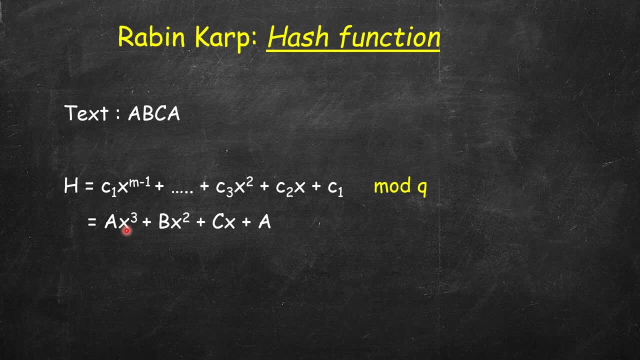 let's say any prime number, let's say 11 and a, b, c, a will be the their sky values 65, 66, 67 and again 65 and modulo q. so in this case there will not be any overflow. but let's say q is some value. 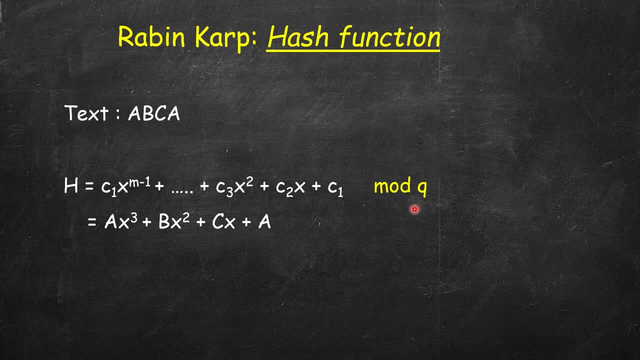 let's say 128 or or some value. so this is how we can calculate the hash function. now let's say we calculated the hash function of some window and we slide by one step. how we will update this hash function in the constant time. because if we are not able to, 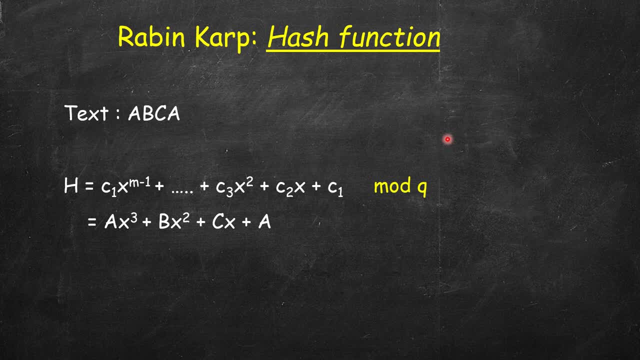 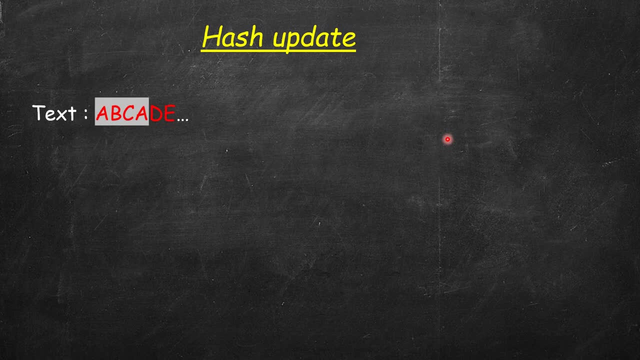 update the hash function in constant time, then our expectation of o m plus n will not be valid. so we have to update it. so a, b, c, a is the window for which we have already calculated the hash. next we slide it by one step. now it's b, c, a, d. so three characters remain same, one character added. 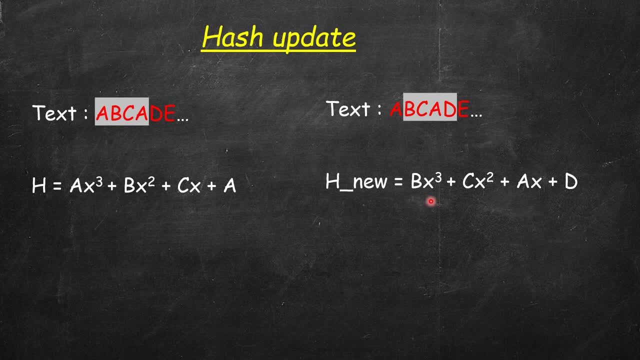 one character subtracted. so new hash function will be b x cube plus b c a d. so we have to update it: b x cube plus b c a d plus a x plus d. now if you compare these two h and h new, you will see that 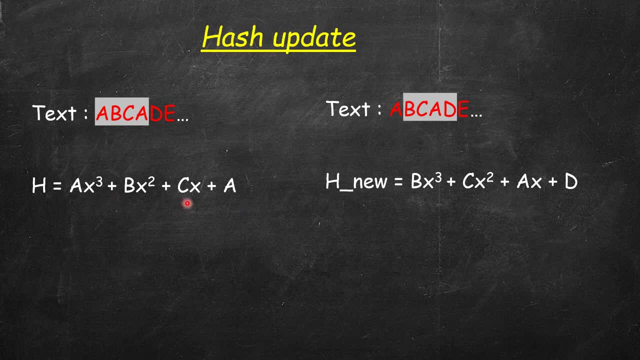 here last three terms are b x square plus c, x plus a. and here you see that first three terms will be similar: b x- cube plus c x, square plus a x. only difference is that one x is extra in all of these three. so if you multiply the last three terms by x, you will exactly get the first three. 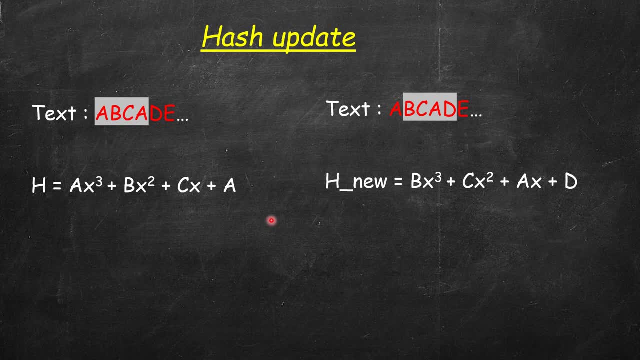 terms of the h new. so what we did here, we subtracted the first value, a x cube. so from h subtract the first value. first value will be always the character that we just skipped, multiplied by x, raised to the power m minus one. so we subtract that value, h minus a x cube. that is constant time then, whatever is. 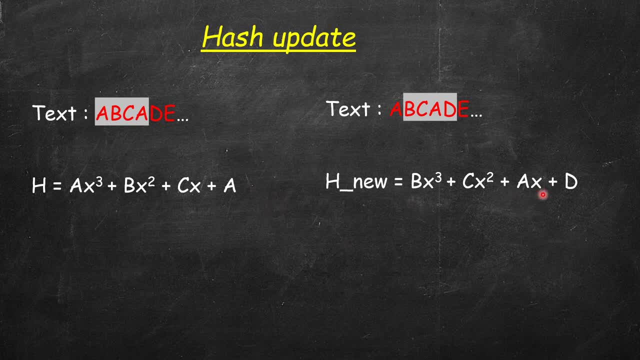 remaining. multiply that with x so we get the first three terms, and after that just add the newly entered character d. so there are three operations: one subtraction, one multiplication and then one addition and of course modulo operation in the end, so it will be independent of the size of pattern. so we can 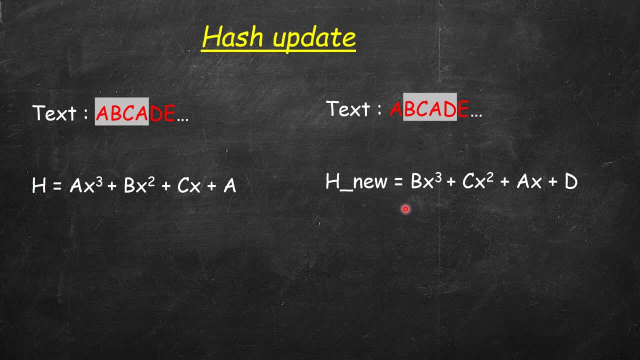 given h, we can calculate h new in constant time, o of one time. so this is what we are doing here. i have not written modulo q, so that is understood. you have to add that while writing the code. now we know how to update it. now let's 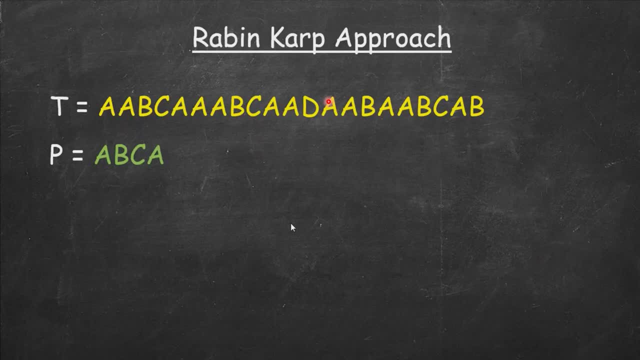 see ravenkarp in axiom. so we have one text, we have one pattern and let's define a simple hash function, not the one we talked. but for simplicity let's say we have a hash function where we just sum the sky values, no more calculation. of course this is not a good hash function and even for 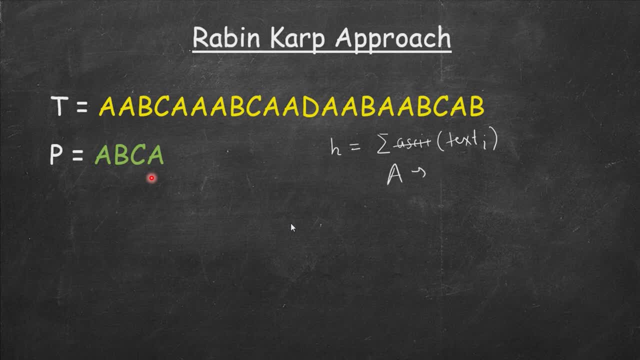 simplicity, let's skip the sky value. also, we will just take a as one instead of 65, 66. it will be even simpler: one, two, three and so on. then the hash of this will be one plus two plus three plus one, one for a, two for b, three for c and one for a, so it's seven. now we calculate the first four characters, hash and it. 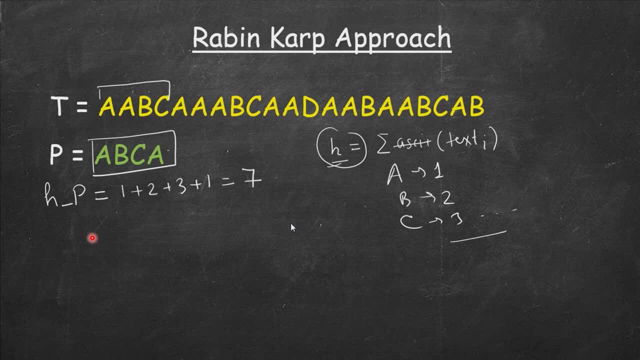 will be also seven, because we add one plus one plus two plus three. so straight away you see that hashes match, but the character does not match. their order is changed now. if there is a match, we do character by character match, but it will not match. now let's move to next window. again it's seven, but this 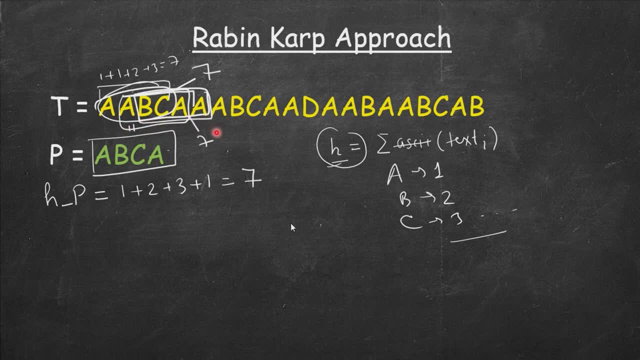 time there is a match, for the next case it will be again seven, but again mismatch. then, uh, next window will be c a, a, triple a, and this time it will be six. so hash does not match, no need to come compare. next it will be a, triple a, b, and this time it's five. again does not match seven, so no need to. 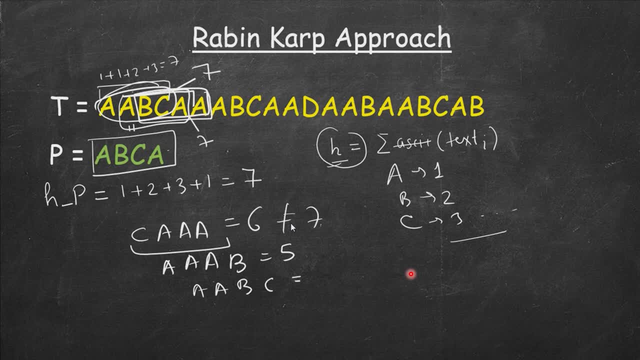 compare. then again there is a match, but character by character shows mismatch. so of course this was a very bad function- hash function. there were many more collisions in our hash function that we just discussed. there will be very rare matches like this. of course this was very poor because just 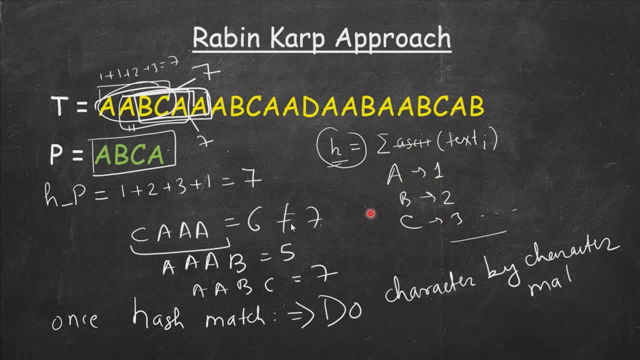 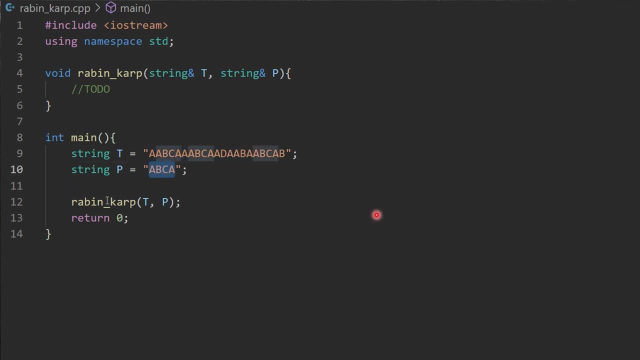 if we change the order it will change. so once hash match, do character by character match to eliminate false positives. now we know how raven carb algorithm work. let's see in our code. so this is the text, this is pattern and we have to define a function, raven carb- which takes text and pattern. 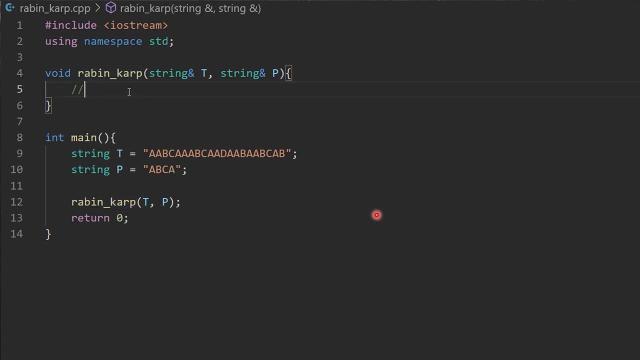 and returns or prints all the occurrences of p in t. so first let's m, denote the length of pattern, then we will calculate the length of text. so n is the length of text, then q is the value. we were talking about modulo, whatever we were taking modulo, and then we had one. 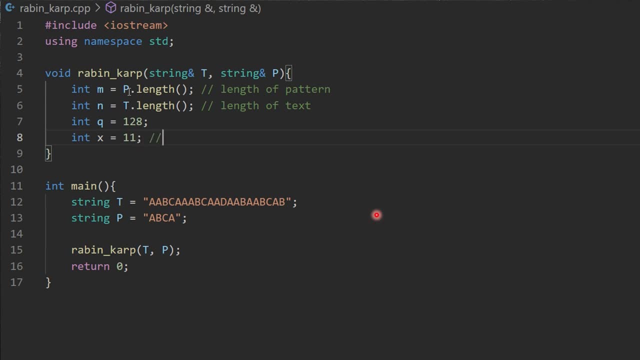 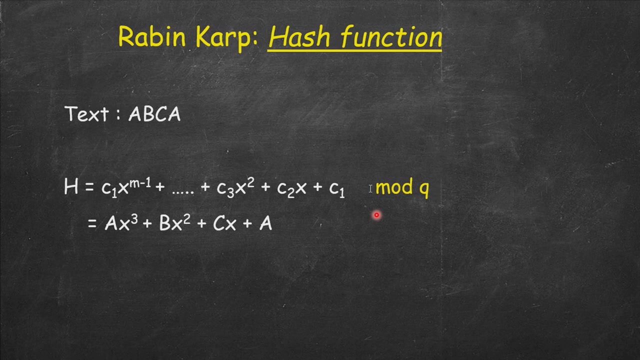 multiplier, if you remember. so we will take some prime value. let's take a small value for simplicity, for easy calculations. if we need to verify, we can verify manually also. so this is the multiplier: x x, 1 x, 2 x cube. so this is the model of q, q term and these x's are the multiplier. we can verify this. 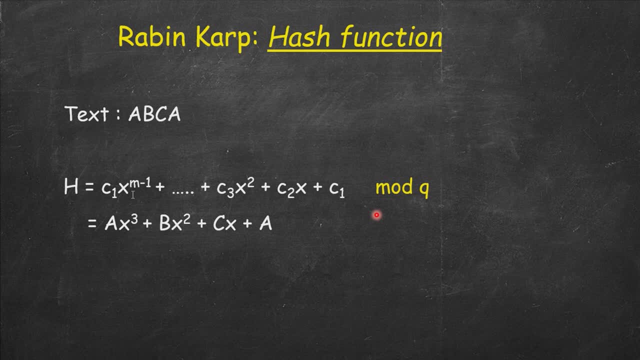 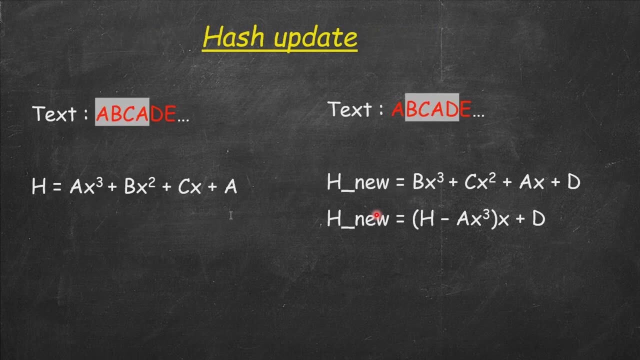 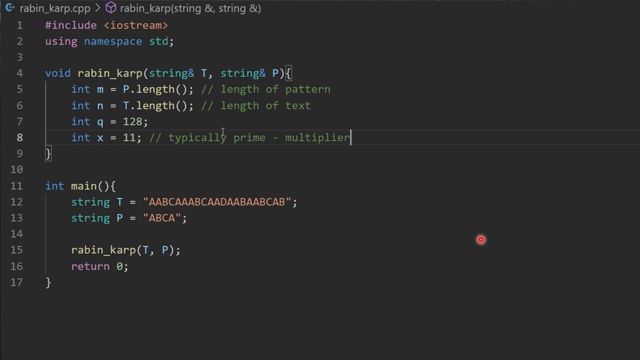 we have just written, so i am writing the same variable name so that you remember now what we did. we subtracted a x raised to the power m minus 1, the first character raised to the power x, multiplied by m minus 1, and then added d, so we need x raised to the power. 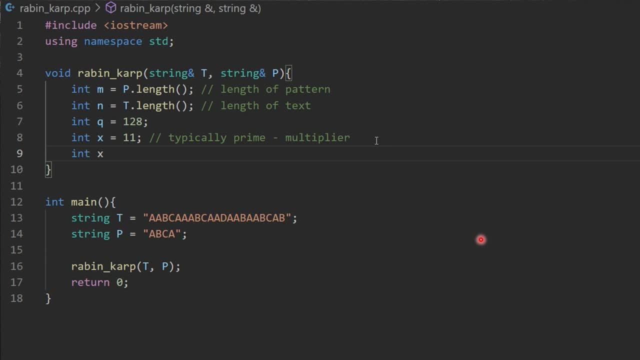 m minus 1, and we will always need that only no other power of x, but whenever we are subtracting. so let's denote it by x underscore m. actually it should be m minus 1, but let's say it's x underscore m. so this will be used for next hash. we have to subtract this quantity multiplied by the. 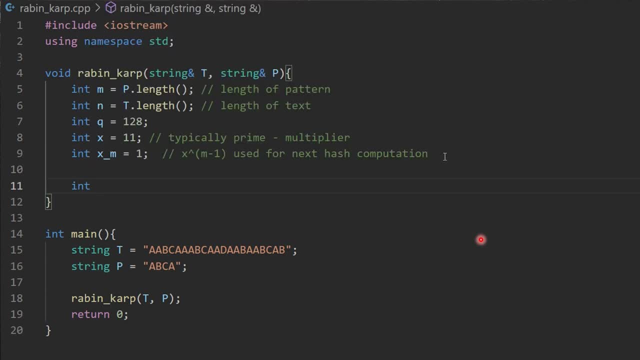 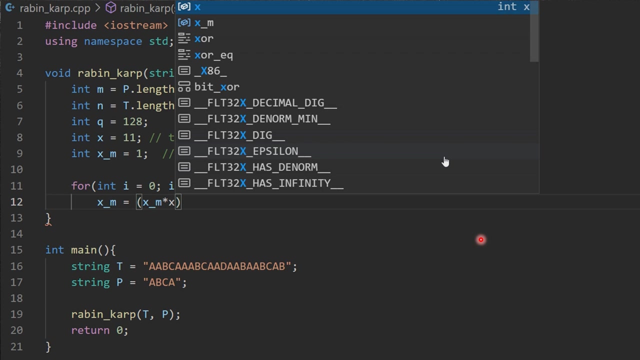 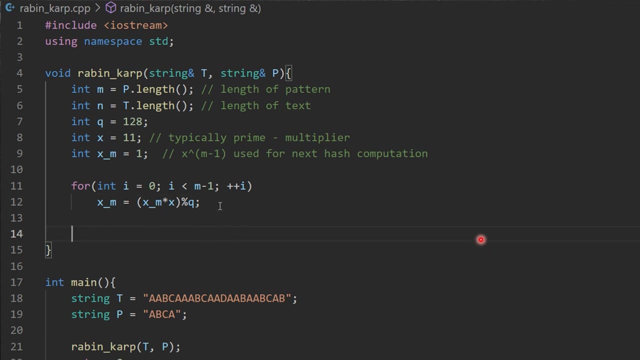 character which is going out of window. so, uh, we can uh calculate this x m. we have to multiply x m minus 1 times and we will keep taking modulo so that it remains within some range of little less than m, like this, after solve this problem, that the input value falls shifted. 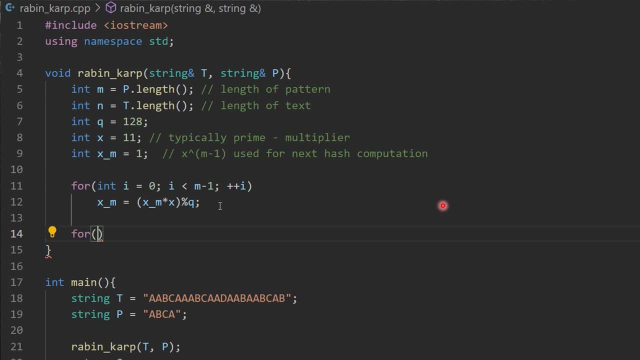 so we have对 allrepresented hash values that we need to see a few minutes later. and now let's calculate. uh, the hash values of pattern, for the pattern pattern is not changing, so we will need to calculate the hash value just once for the text we will be updating. so let's calculate the first window. 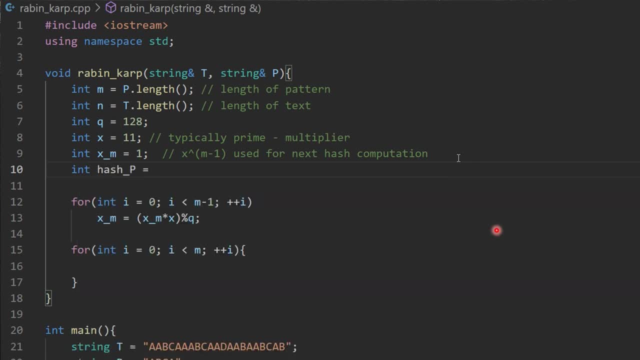 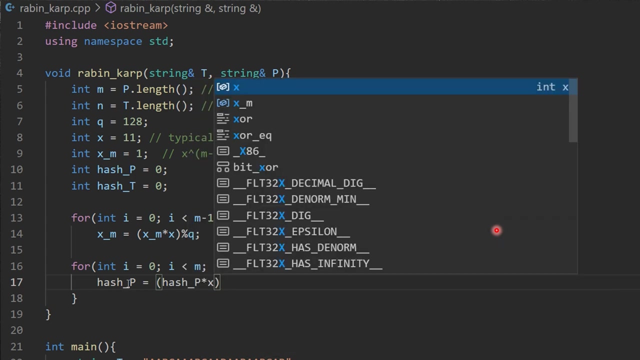 capture them in hash underscore P for hash of pattern and hash underscore T for hash of current window in the text. so initially we are just calculating the hash of pattern and the first window of the text. since both are of length M and similar calculation is required, we can club them together under one loop. 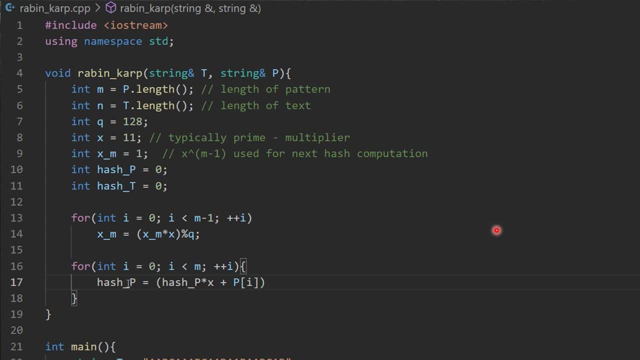 in the next loop. so what do what we do? we multiply by X, add the current character and take Modulo. in the next time, when we multiply this whole thing by X, you will see that whatever was X here becomes X a square, and so on all the way up to x, to the power M minus 1. similarly for text. now we have first. 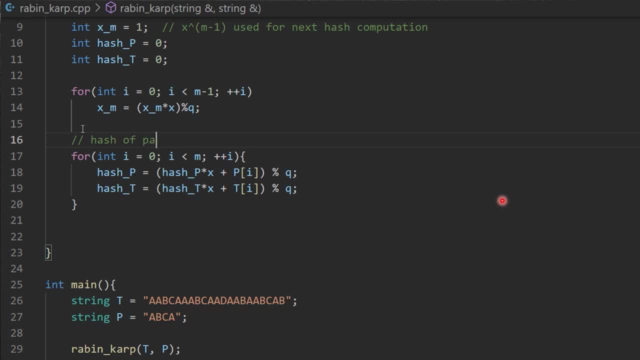 window and and hash of the pattern. now we will start matching and updating the hash within one loop. so we will start from 0th index, 0, i equal to 0 and we will not go till n, but we will stop at the start of last window and last window will. 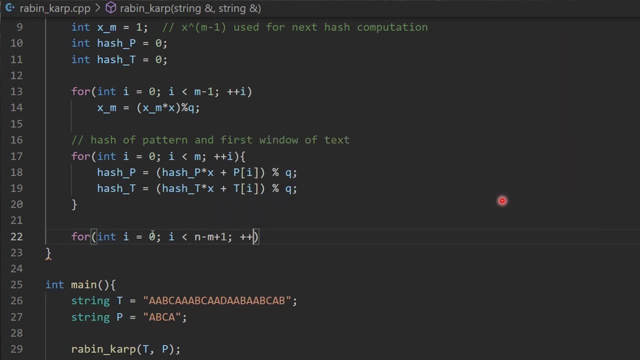 stop at n minus m. so we will be checking till it's less than n minus m plus 1. for example, if n is 3, let's say text size is 3 and pattern is of size 2. so there will be just one slide, compare in the beginning and then slide by one step. so 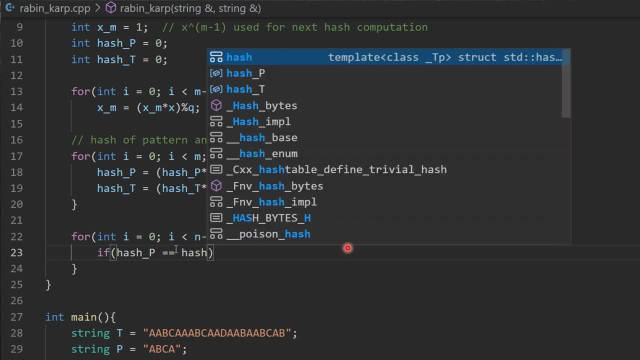 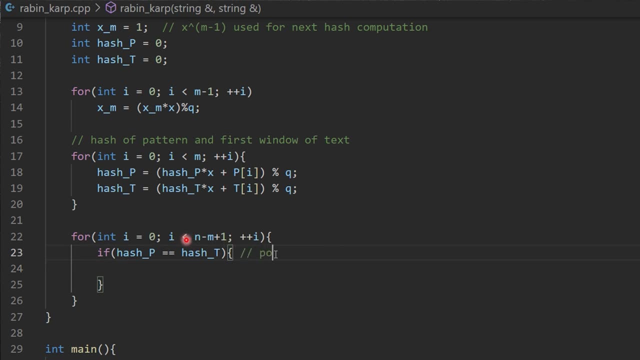 the starting index for that will be 1. so you can see, 3 minus 2 is 1 and it should be 1 and it should be one times only. so that's why, since we are taking less than we are adding, plus one if you are taking. 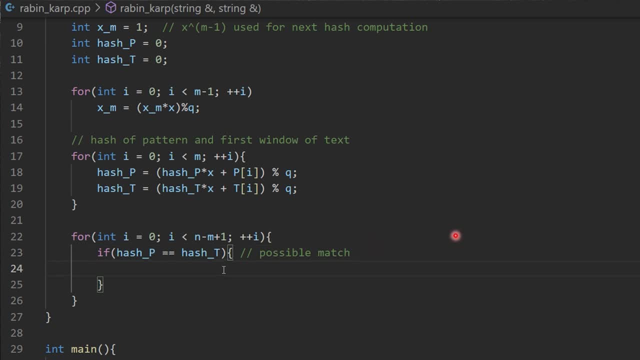 less than equal to, you can remove plus one. so if the current window hash in the text matches with hash of pattern, there is a possibility of match. there is a chance of match. there is a high chance of match if your hash function does not. for your hash function there are not multiple collisions. 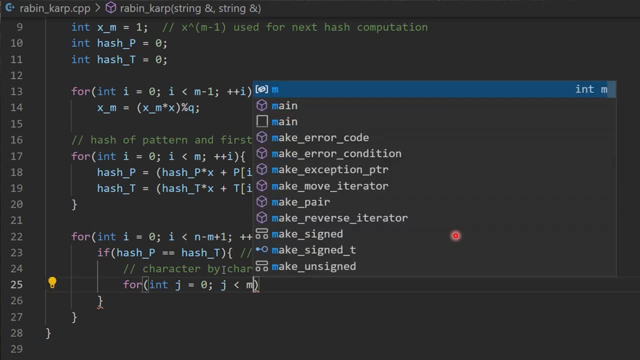 but if your hash function is poor then there is a kind of 50: 50 chance. in our case it will be very high chance. there are very less chances of collision. now we will do character by character match to make sure that we don't include any false positive. so there will be, in the worst case, m. 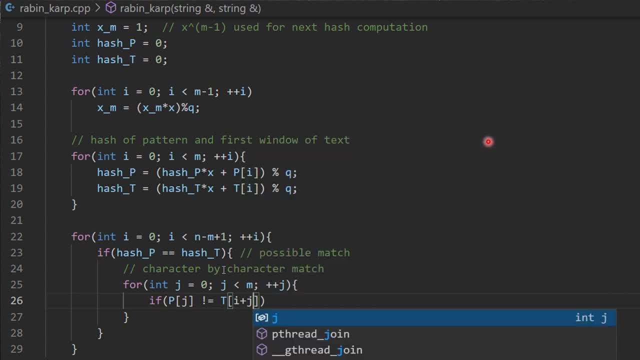 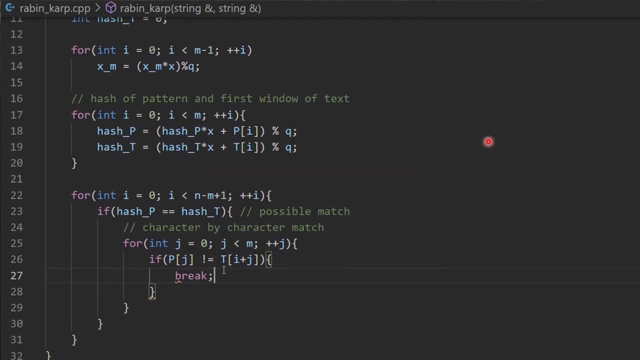 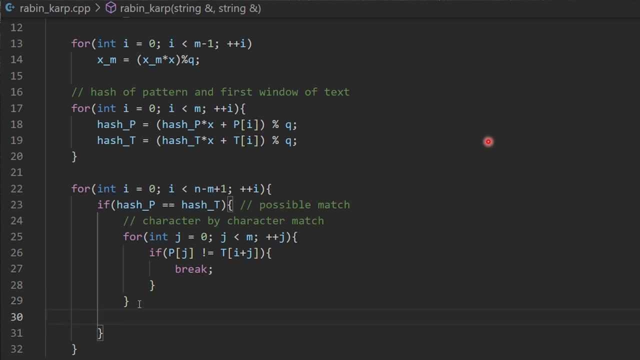 comparisons. so this loop goes from 0 to m m minus 1 and p of j. if at any point of time we find mismatch, then we break. no need to compare further: we found a mismatch. but if we did not find any mismatch in this complete loop, then that means there was a match. so we will return. 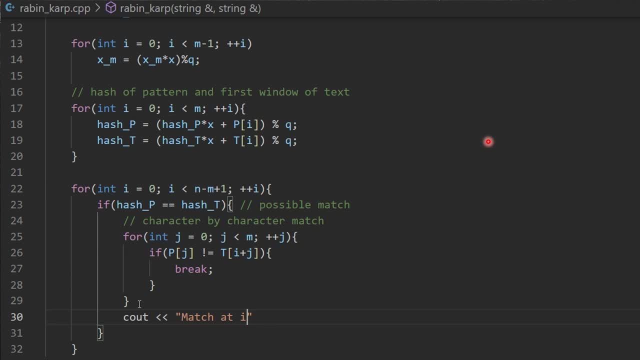 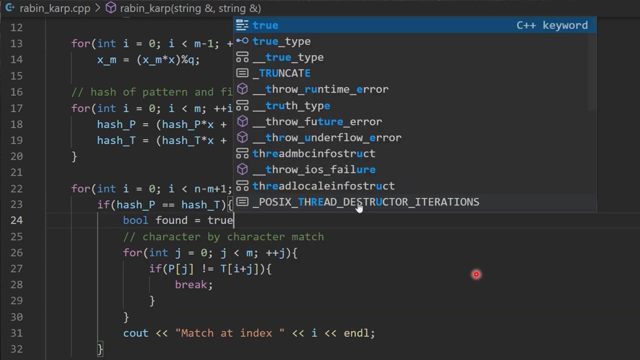 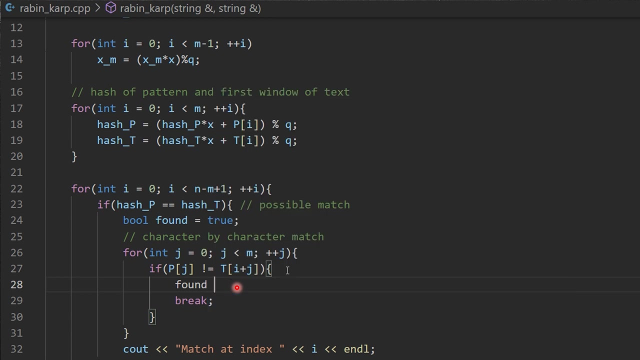 match found at index. whatever is i, but this will currently execute, irrespective of break or not. it will break and it will print. so we will keep a flag found and we will make it false just before break. so bool found is true by default. if this break condition did not hit, then it will remain true. otherwise we will make it false and we 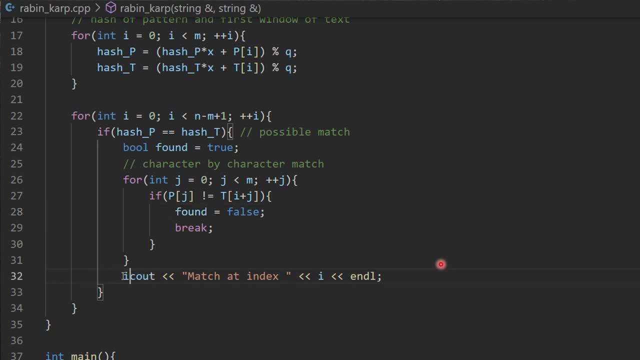 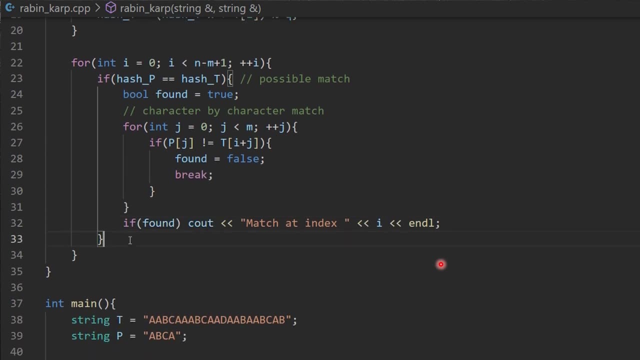 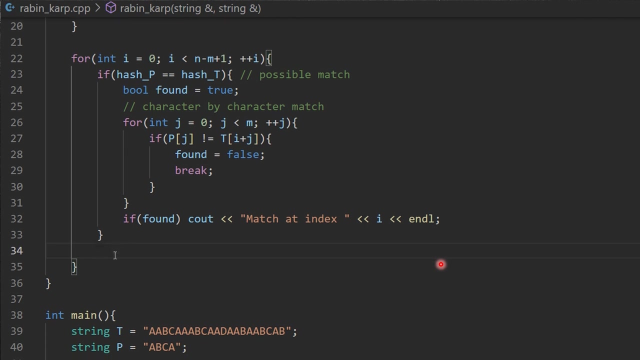 will print this match. found only found is true. so now this is for when the hash is matched. we have other condition: hashes does not match, then we have to calculate the hash of next window. but we have to make sure that this was not the last window, if this was already the 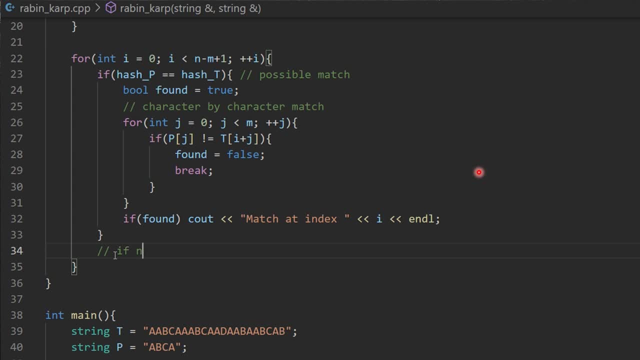 last window and we did not find any match, then no need to compare further, no need to calculate the next hash. we have already compared the hashes for the last window. so if it was not the last window, then continue hash computation. so what is the check for that? if i is exactly equal to n minus, 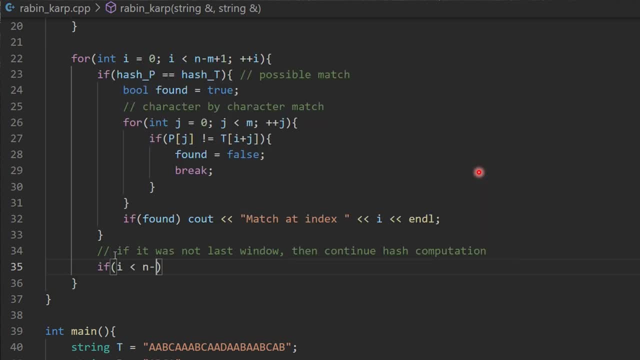 1, then this is the last window. so we have to continue this only if i is less than n minus m. so hash t, and you know how to calculate hash t. so whatever was old hash t minus. remember that x raised to the power m minus 1, multiplied by the character that just. 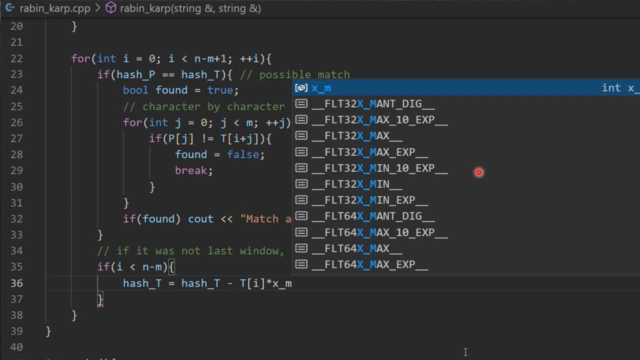 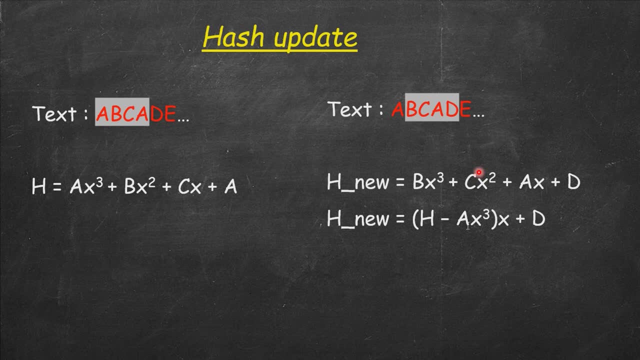 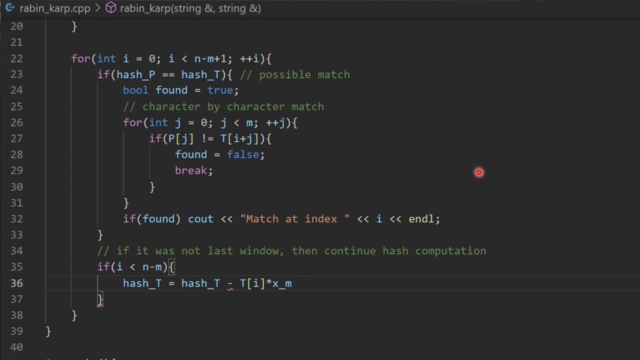 went the leftmost character in the previous window. so here a. a went out of scope, out of window. a multiplied by x, raised to the power m minus 1. so this is what we have done here and now we multiply the whole thing with x, the same multiplier, and then add d, the new character. so multiply whole thing with x, so we are. 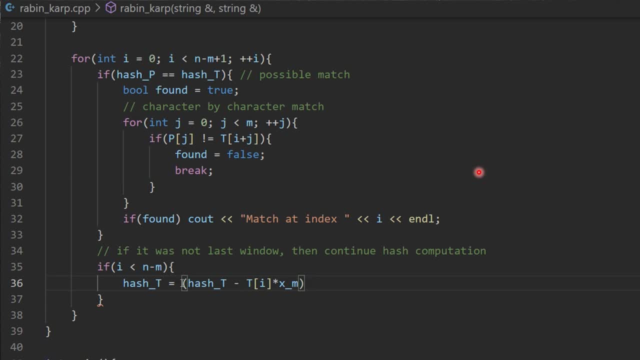 just following what we saw in the explanation. if at any point of time you are lost, go back to the slides, see how we calculated it and then write your code accordingly. then we add the newly introduced character, which is t of i plus m, and then don't forget to take the 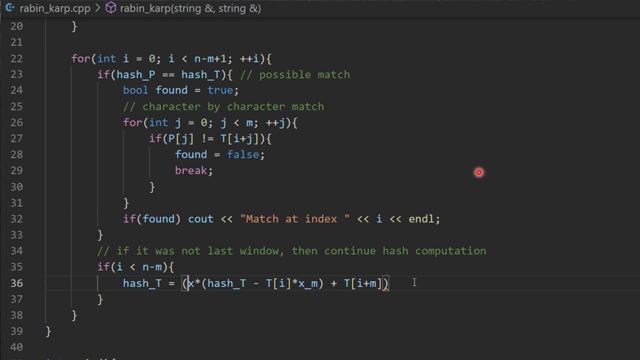 modulo q at each step and one thing you can notice is that this hash t minus t i multiplied by x raised to the power m minus 1. this can be negative because this x raised to the power m minus 1 can be a large quantity. so minus this. 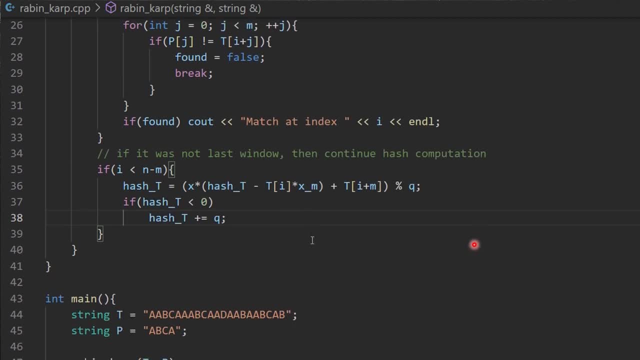 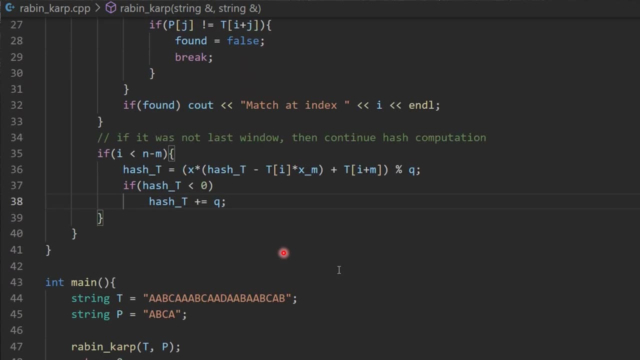 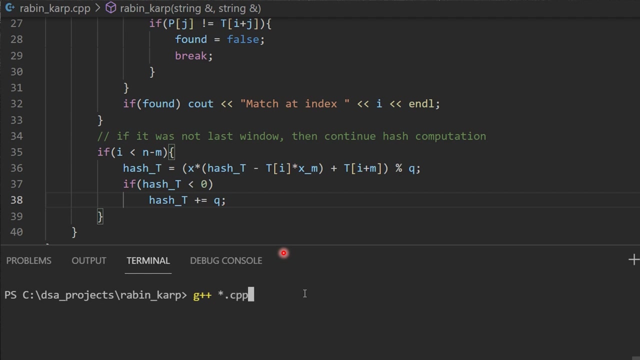 can take this value negative and take modulo of negative, it will be negative. so if it's less than zero, just add q, because modulo q it will not be less than minus q. so adding q should make it positive and we are done. so let's compile this now and let's run this. and it found three matches. 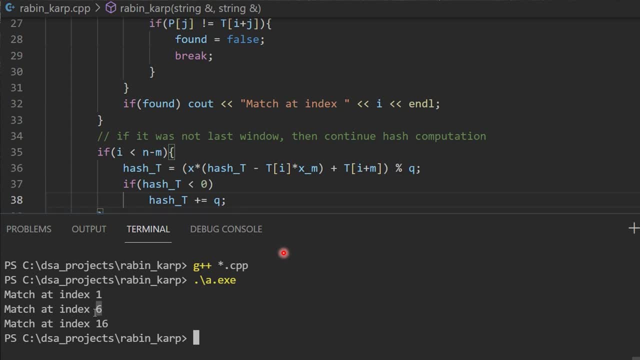 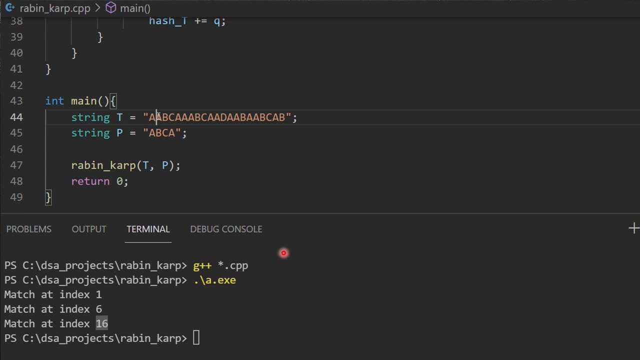 at index 1, that is second character, and it found three matches at index 1, that is second character, 6, that is seventh character, and 17th character 1, 6 and 16. and you see in this, at the starting second character, there is a match. if i highlight it, you can see it has. the id is already highlighted.